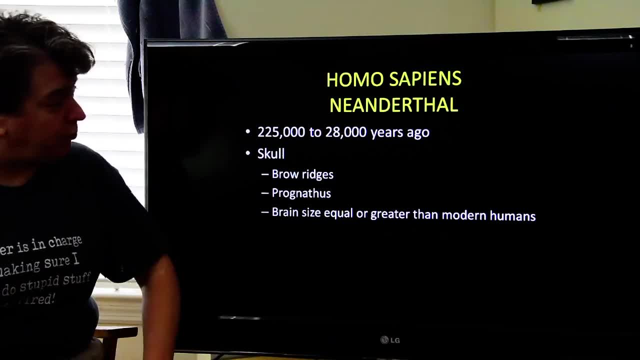 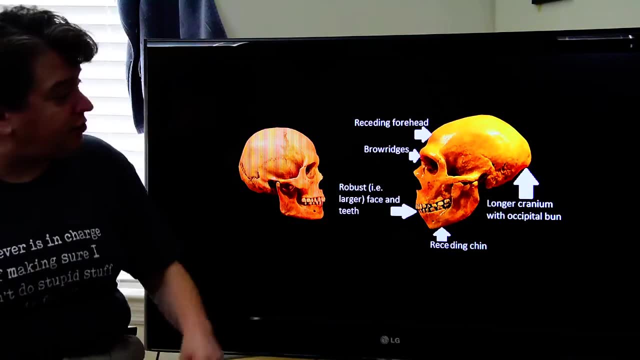 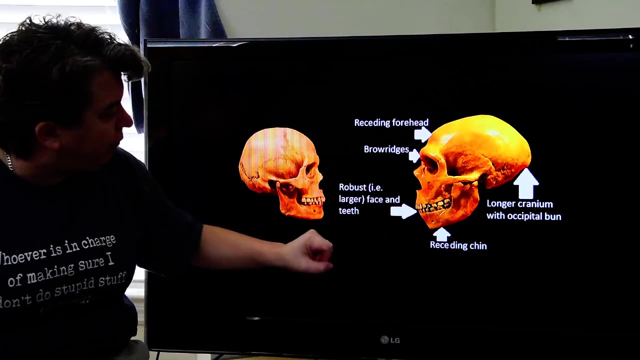 downwards, and their brain size, though, is equal to, or sometimes greater than, modern humans, And so this is the skull of a modern human, This is the skull of a neanderthal, and there we can see some of the differences that you would have. This reseating forehead, the brow ridges. 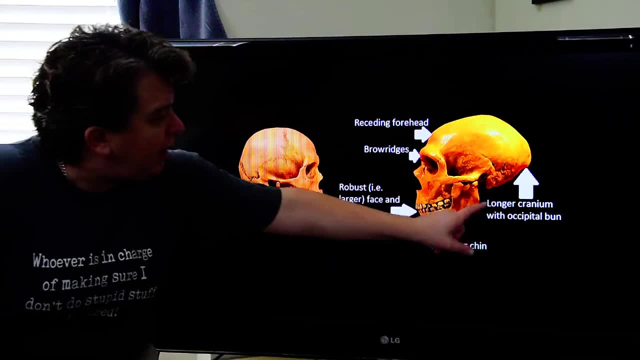 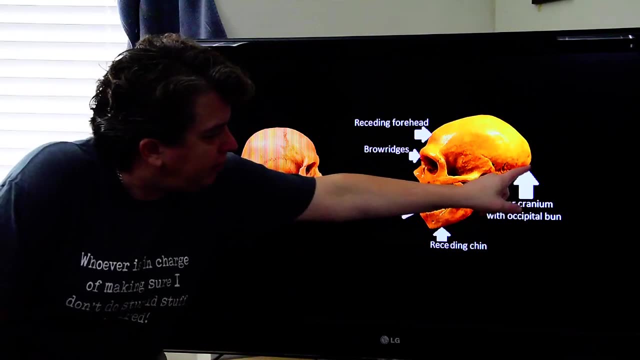 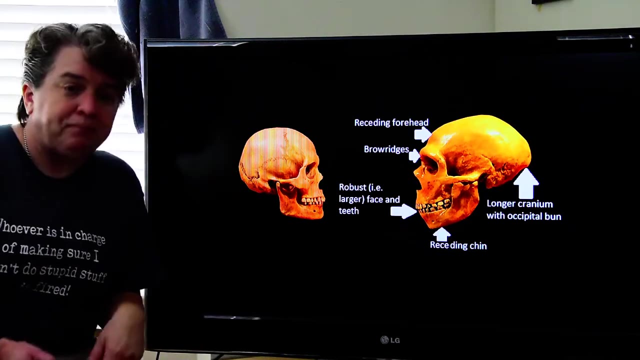 there we have that prognathous chin, and they do tend to have also on the skull this thing called an occipital bun, and this little � endorsement 00 inside the head and chest cats, but not really the back of their skull that we don't see in modern human skulls. 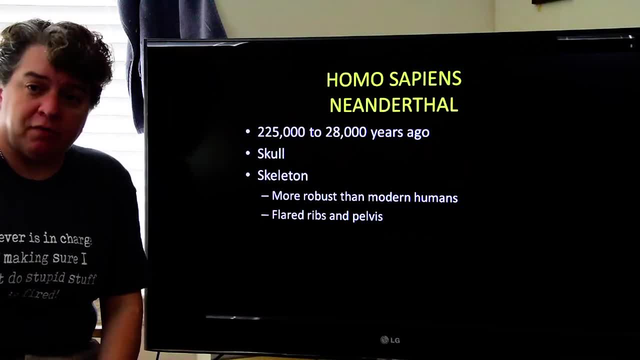 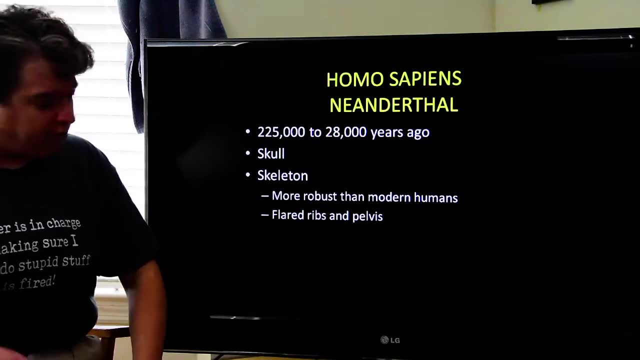 The skeleton of Neanderthal was more robust than modern humans. That just really means that it's kind of beefier, stronger, Has flared ribs and pelvis, and if you would have seen one of these guys, you would think of them as being very sturdy. 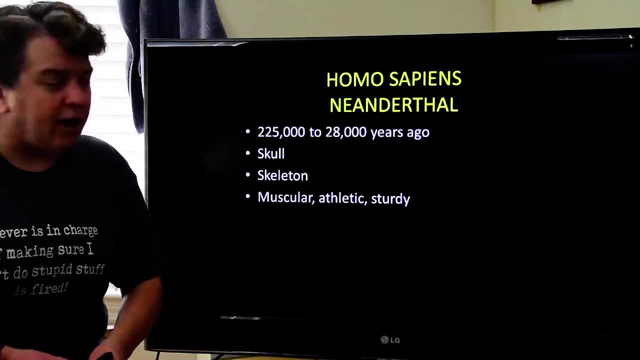 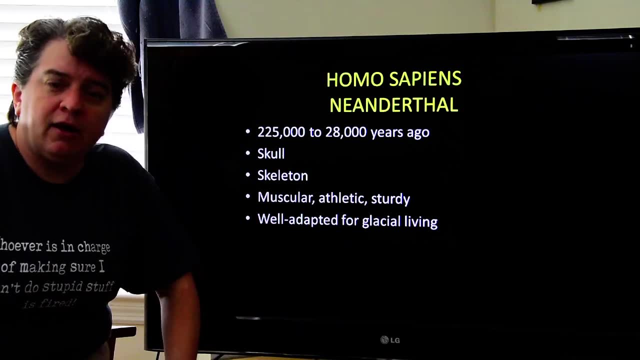 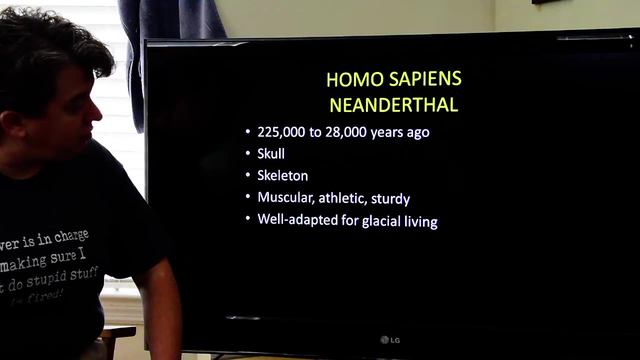 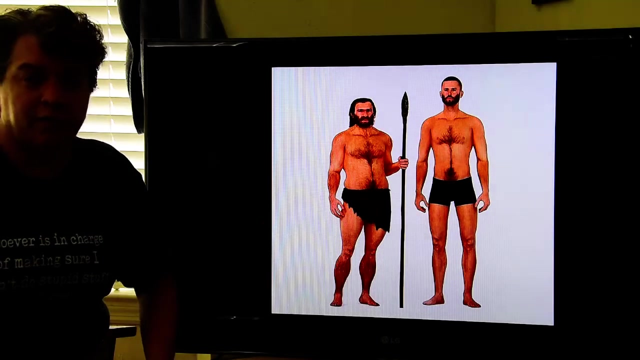 They would be very muscular, very athletic and just very robust. This is good, because these guys lived in the ice age and they were well adapted for living in those colder ice age climates. So if we saw a modern human and a Neanderthal, that's really kind of the difference you would. 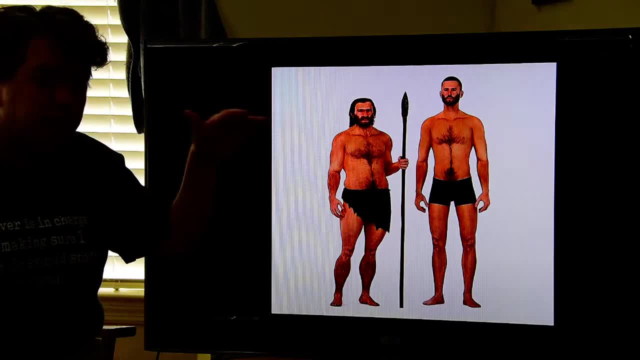 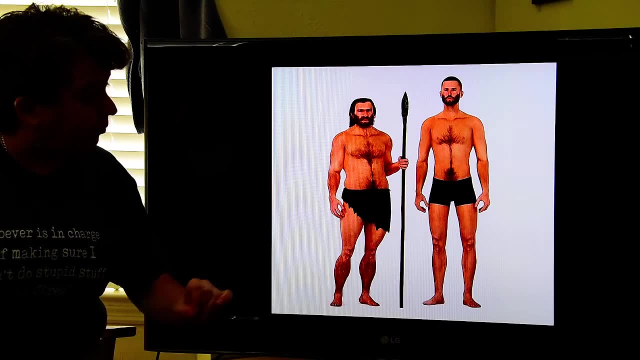 end up seeing, And again, usually a little bit more robust, A little bit shorter, a little bit broader and beefier, But that's good when it's colder, because he's not going to lose as much heat as your modern humans might. 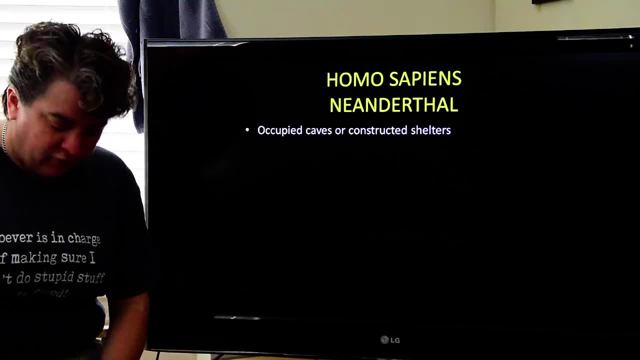 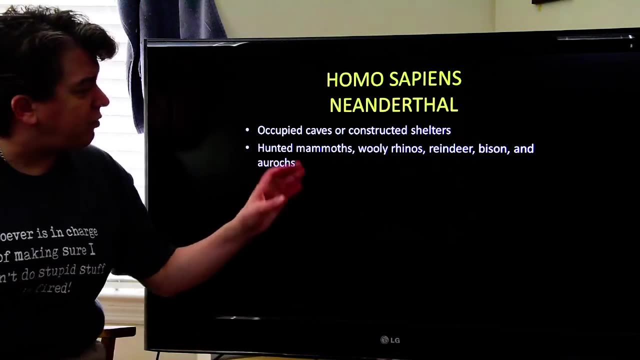 Now, Neanderthals occupied caves or they constructed shelters to live in, And they were very, very good hunters. They hunted mammoths, woolly rhinoceros, reindeer, bison and an organism called the raccoon. 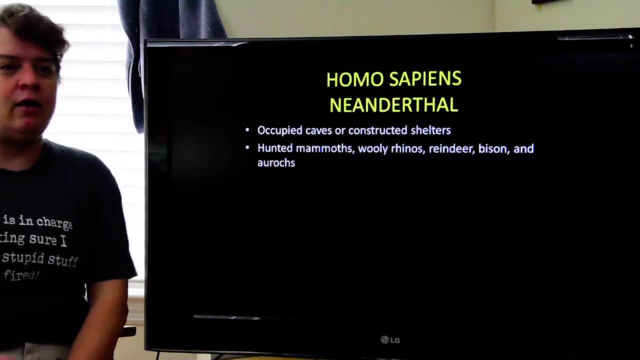 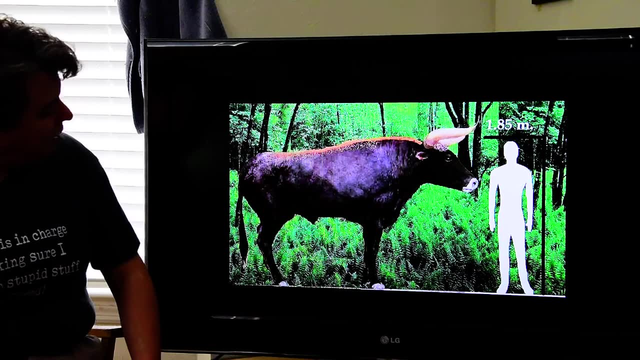 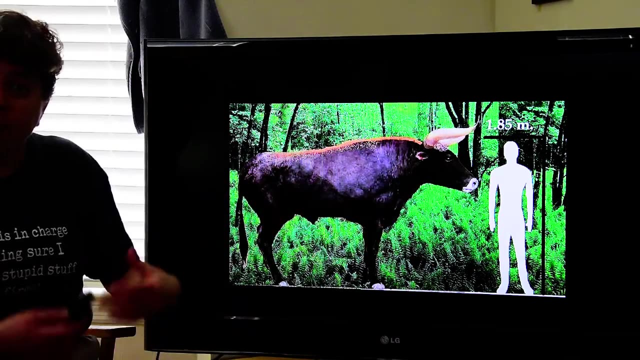 Rhinoceros were also very good hunters- called an auroch, And an auroch is basically a giant cow. So this is what an auroch- the size it would have compared to about a six foot person. So we have like a really big wild cow, These guys. 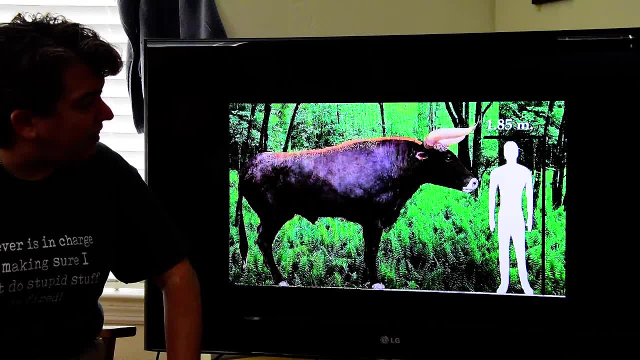 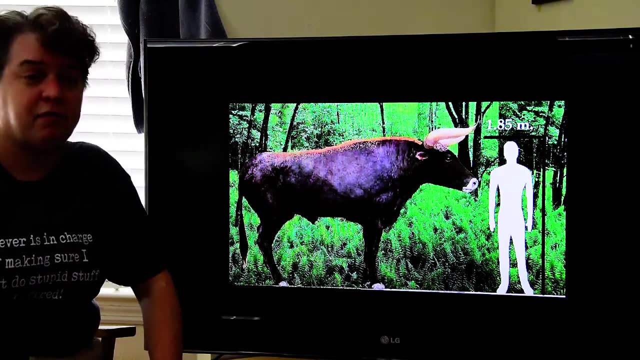 would have lived in the forests of Europe. In fact, the last auroch actually died in- I think it was in Poland in the 1600s, And that was the last auroch alive. So they are extinct now. But these were wild cows that inhabited Ice Age Europe, Neanderthals. they used tools. 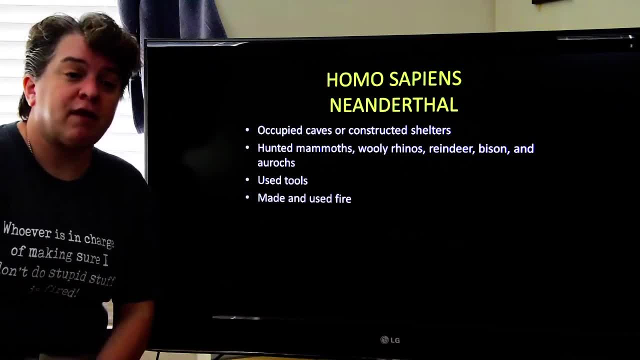 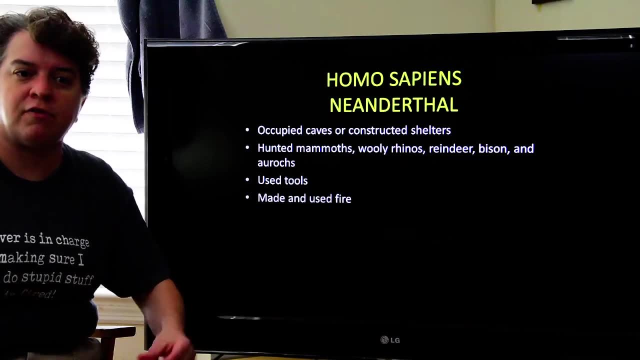 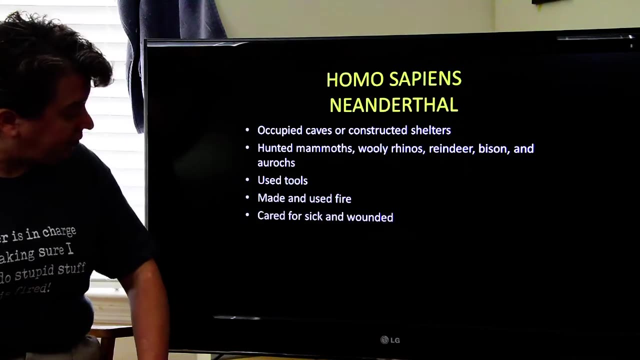 and they made and used fire. And in this case we know that they made and used fire because we do see that repetitive use in these caves and shelters and things. So we definitely know that they knew how to make it and use it. They did care for their sick and wounded And we can see. 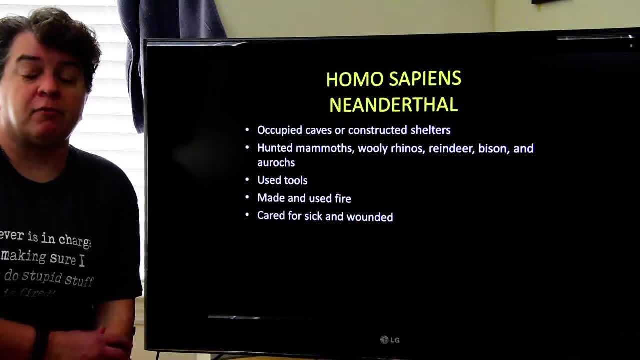 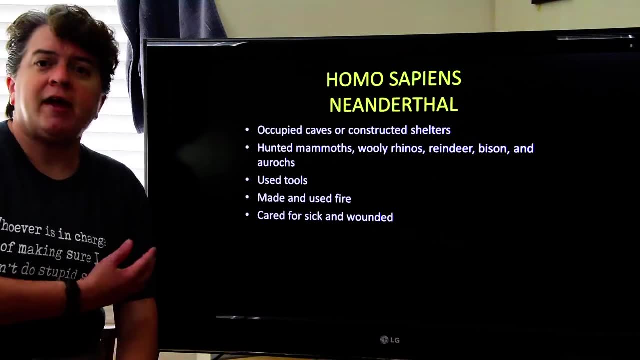 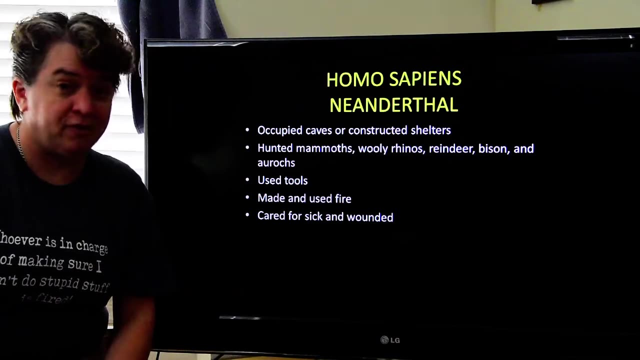 this in the form of, like some really awful injuries that would have occurred when hunting some of these very dangerous animals, And then they healed. Like one guy lost part of the bottom part of his arm And obviously that would you know if he wasn't getting any kind of care. 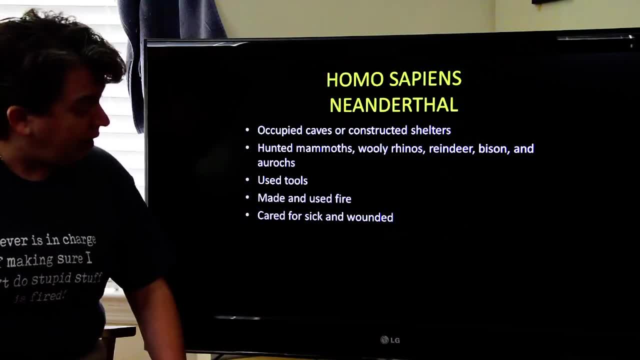 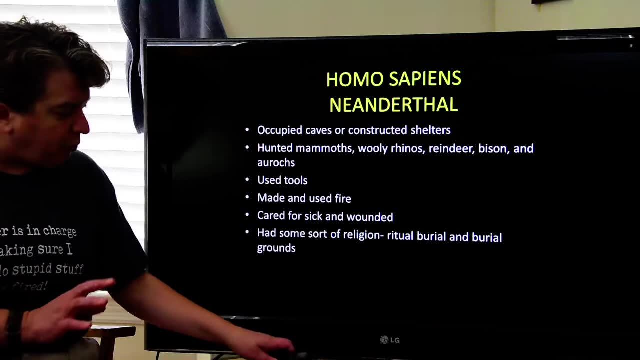 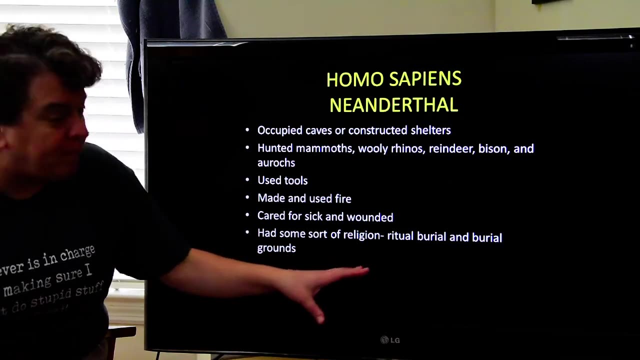 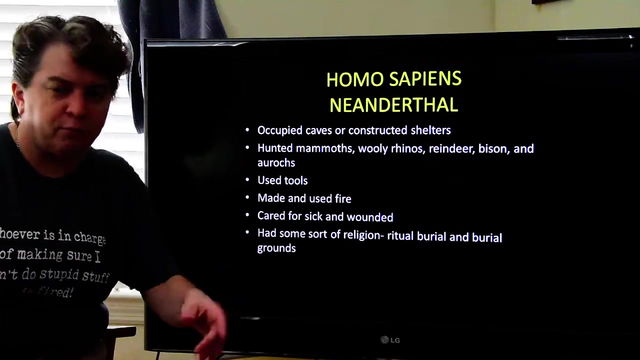 that should have killed him, But it ended up healing, So we know that they did care for each other. It looks like they had some sort of spiritual belief, some kind of religion, Because we do see that they have ritual burials where they would bury people with, like, surrounded by flowers and some tools and things, and 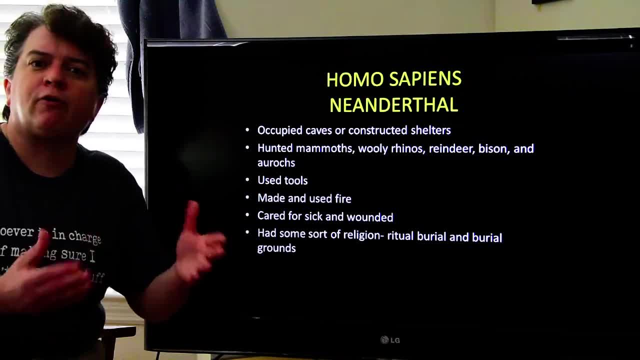 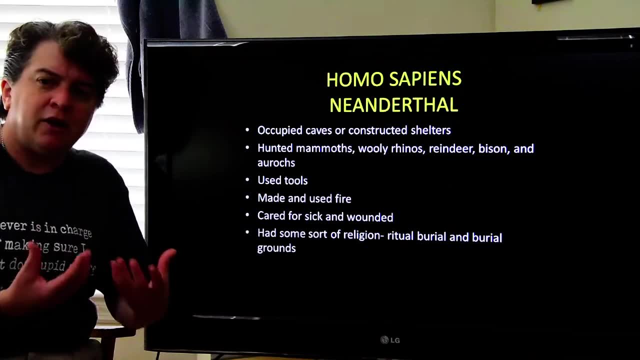 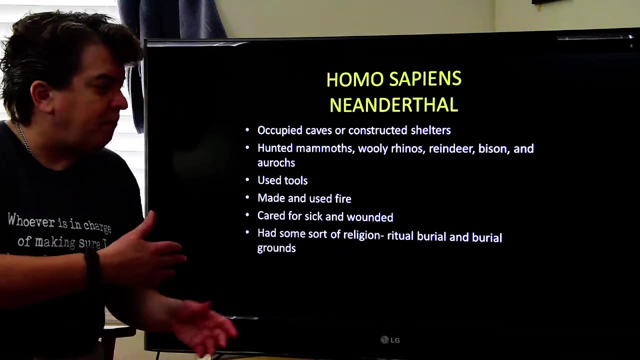 artifacts of certain kinds And they had burial grounds, places where the people were buried, Very specific locations, And so that insinuates that suggests that they had some kind of spiritual beliefs about the afterlife, But of course we have no idea exactly what those would have been. 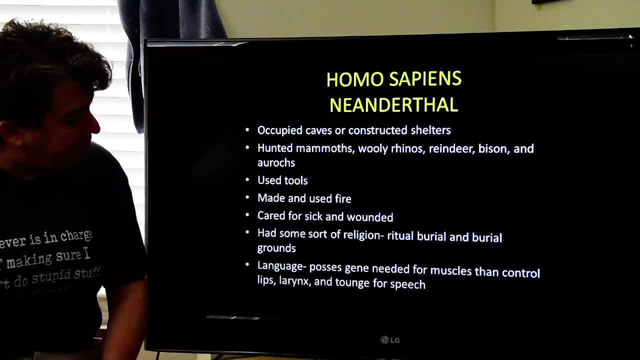 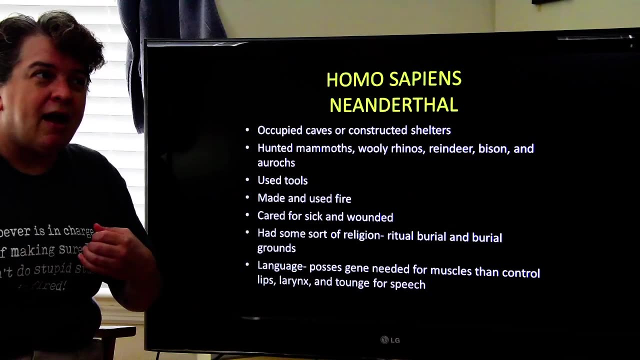 Now, when it comes to language, they, when we sequence Neanderthal DNA, we know they possess the gene that is needed for muscles that control the lips, the larynx and the tongue. So we know that they had the genetic code in order to be able to talk. But, of course, since we 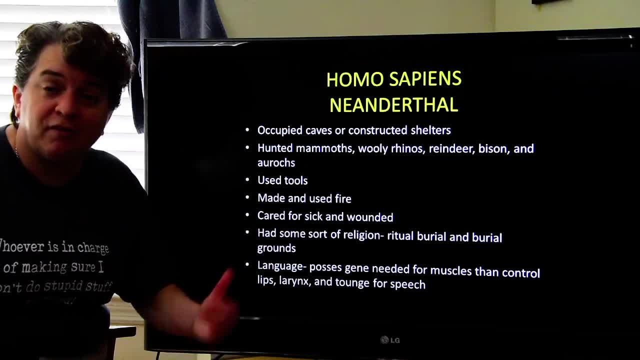 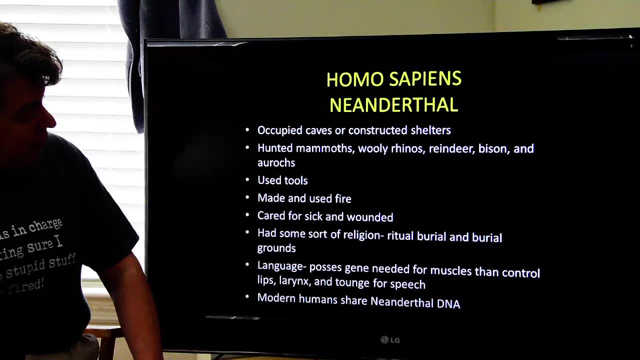 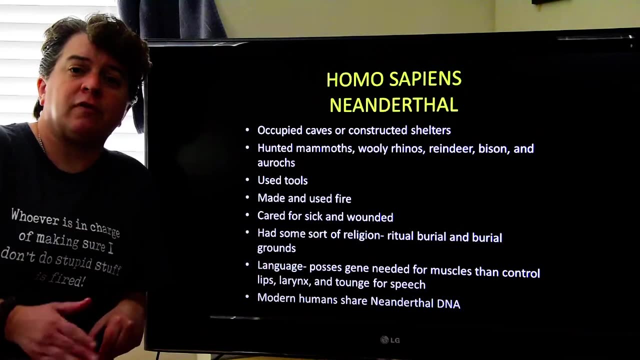 don't have the time machine to go back in time and see these guys alive. we don't know what that speech would have been like Now. modern humans do share Neanderthal DNA, unless you come from Sub-Saharan Africa. So if you're 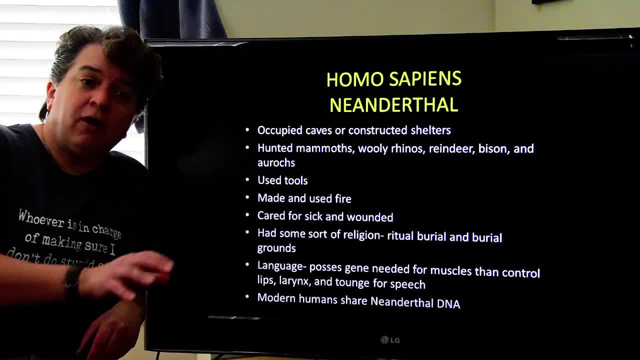 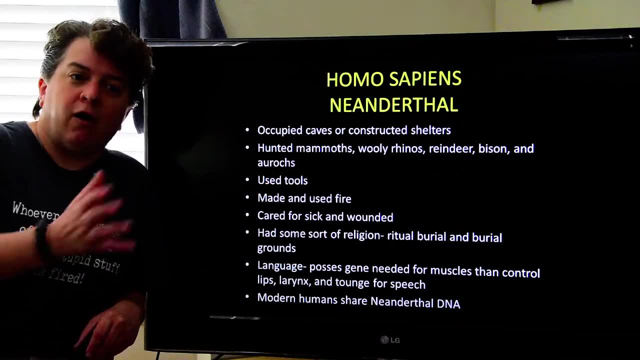 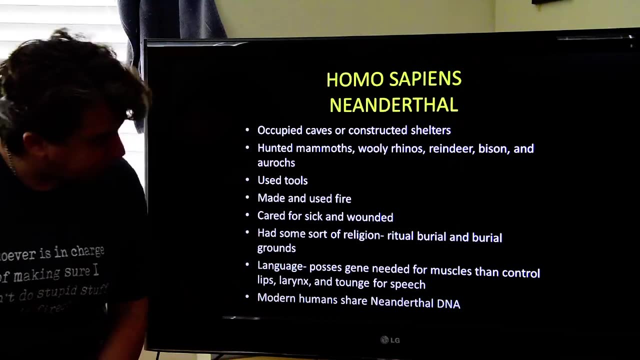 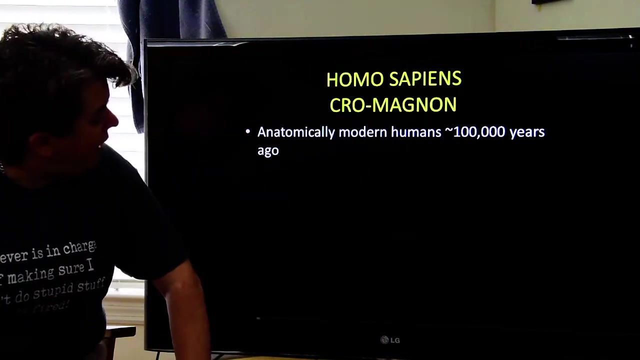 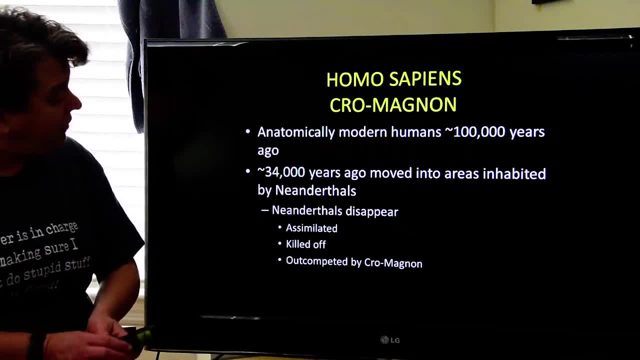 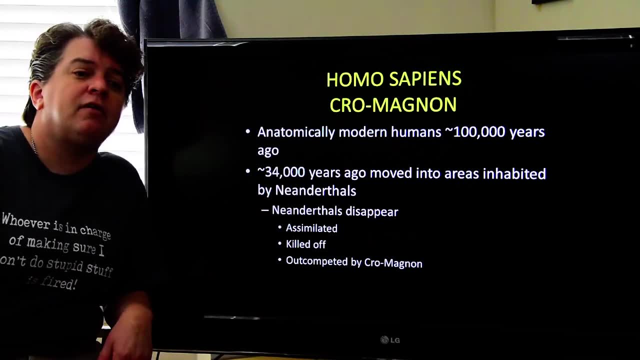 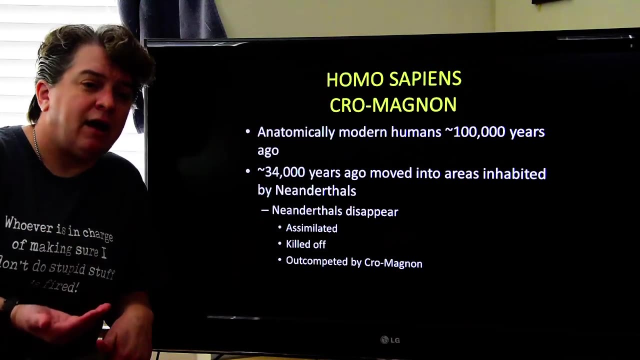 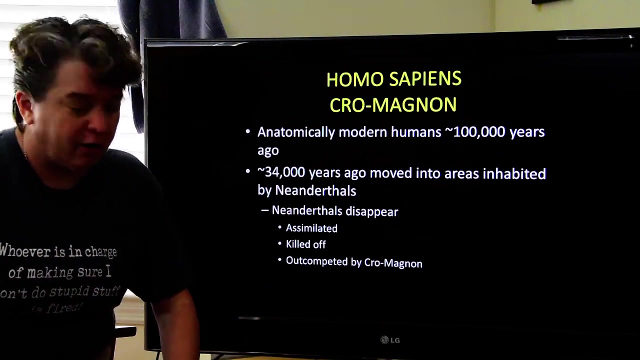 thousand years ago they moved into areas inhabited by the Neanderthals, and after they do this, the Neanderthals disappear. and the question then is: what happened to those Neanderthals? and back when I went to school, the the the night party line, the common thing was: the Cro-Magnons came in and they killed them. all. well, obviously they didn't kill them all if we have some Neanderthal DNA in us right? so nowadays we're looking at where the Neanderthals assimilated, meaning did they just sort of mix together with the Cro-Magnon and that's. 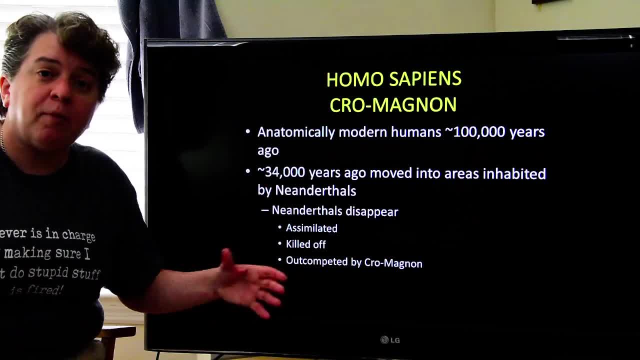 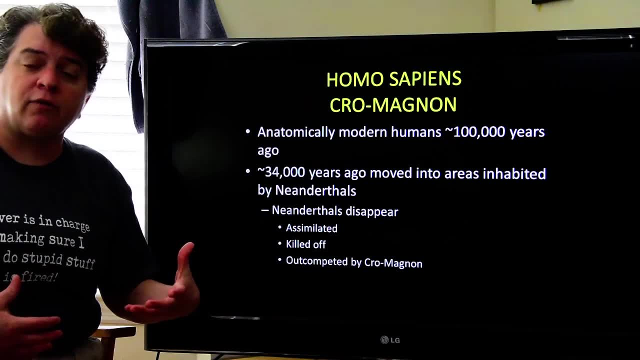 why they disappear or were they out-competed by Cro-Magnon? meaning, as the Ice Age is coming to an end, having those Neanderthals and Cro-Magnons in the Neanderthals and the Cro-Magnons in the Neanderthal characteristics are no longer as advantageous as having the 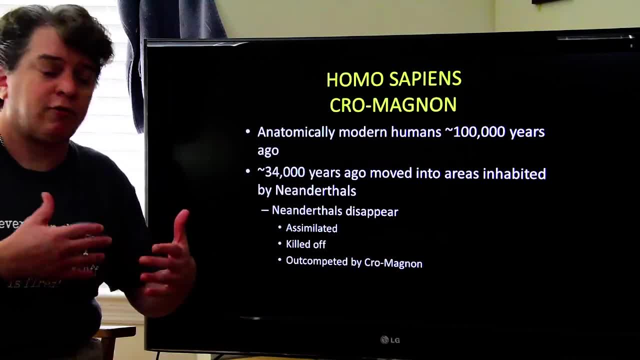 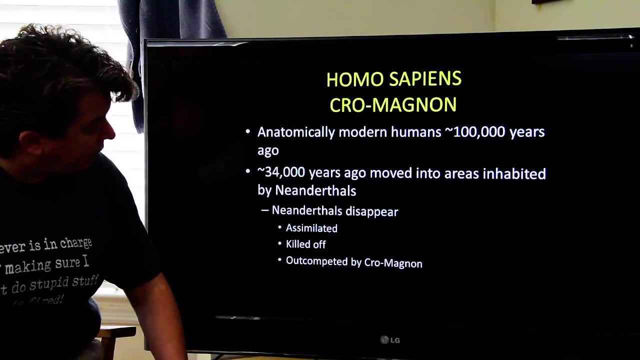 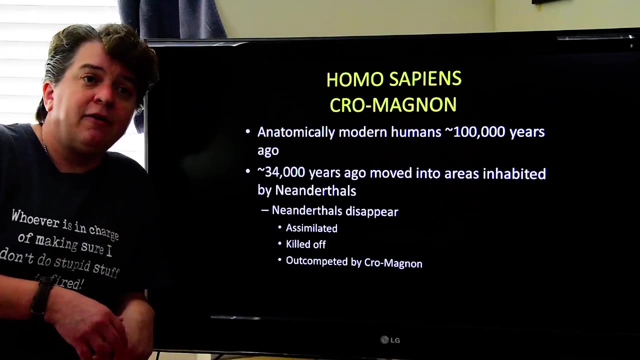 modern human characteristics and so, basically, Cro-Magnon was able to out-compete them. well, I'm sure, in reality, what we're really looking at is some of all of this, since we carry Neanderthal DNA. definitely, you know, there was some assimilation. certainly, some were probably killed. 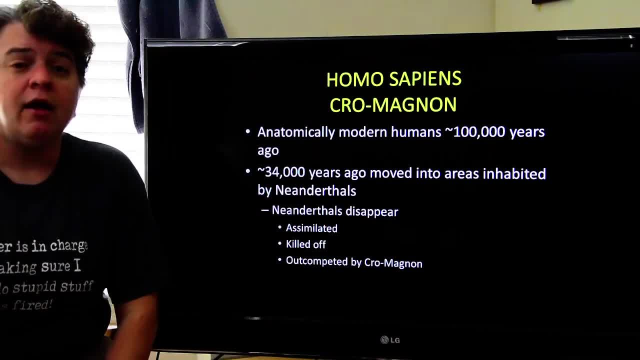 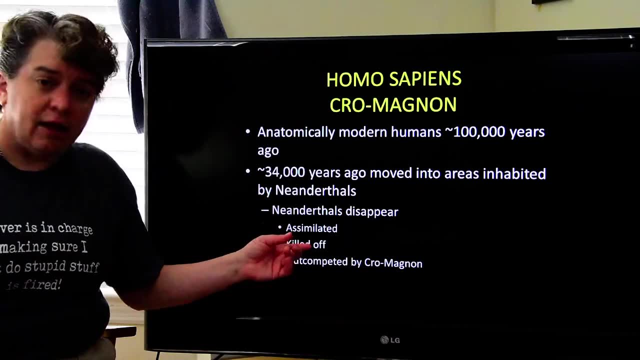 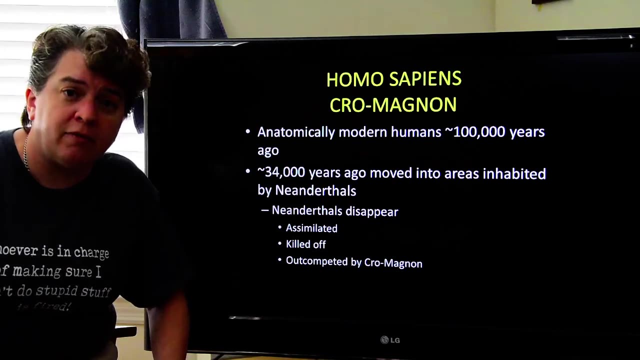 off, I would imagine. just like in modern days, you can have different groups of people inhabiting the same area and they're gonna fight over resources, and so I'm sure some of that happened at this time as well, and as the climate was changing as we are coming out of an Ice Age and surely things Cro-Magnon was. 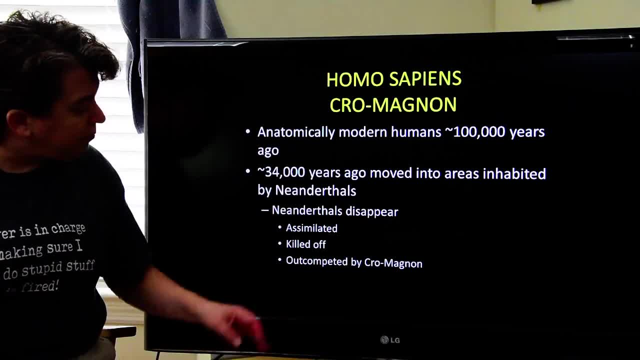 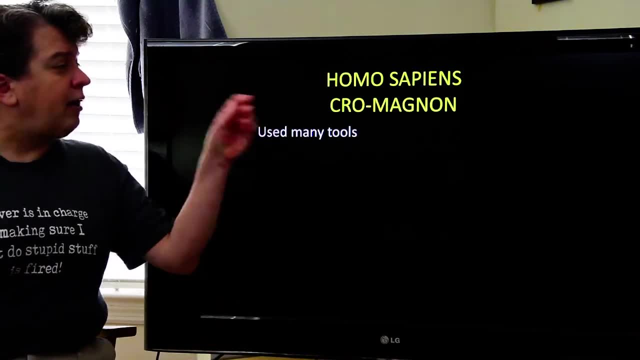 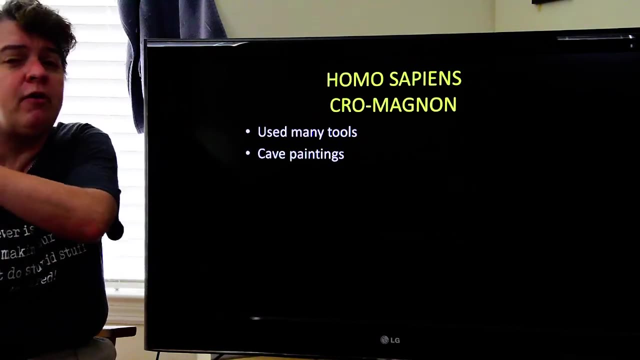 able to out-compete them for resources as well. so it's probably not one single one of these things, but all three of those things occurring at that time. Now, Cro-Magnon used many tools, very, very talented tool makers, And also they had quite a bit of artwork. 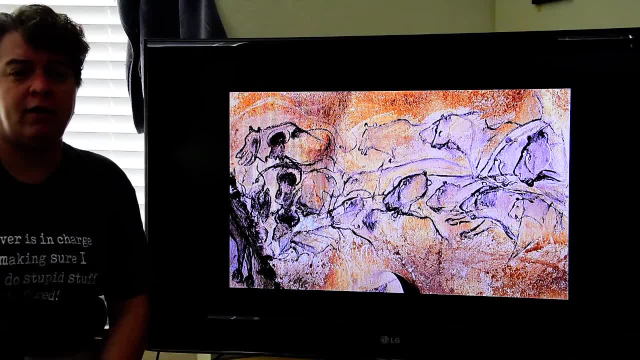 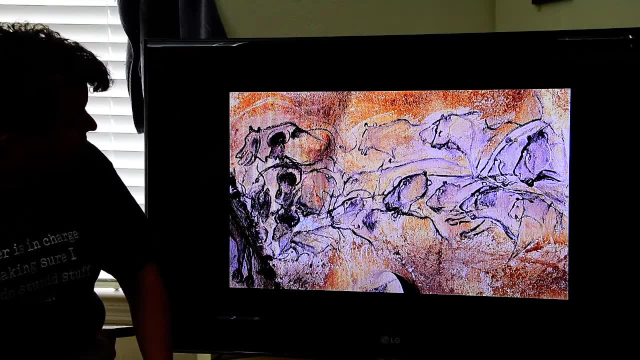 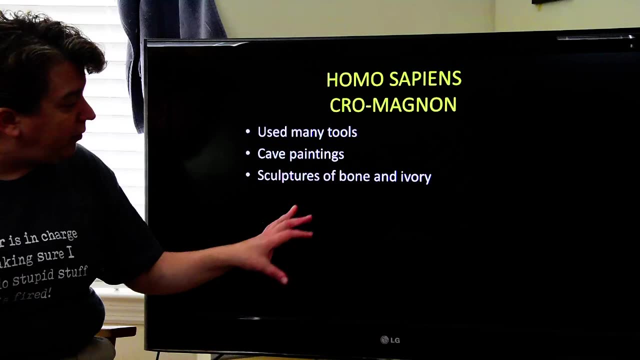 There are numerous caves in Spain and France and other places where we can see some of the artwork that was done by these early people. They also made artwork by sculpting things. They would use bone and ivory and carve shapes- often human shapes, in these ivory pieces and bone pieces. 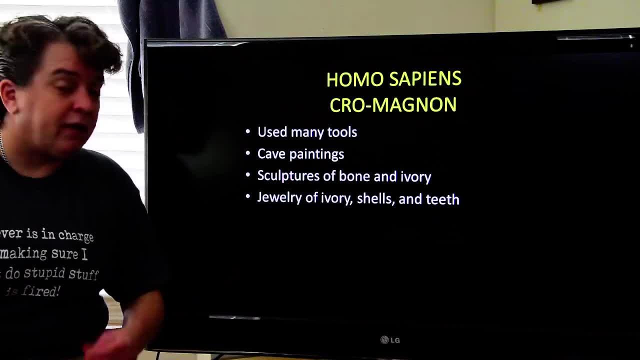 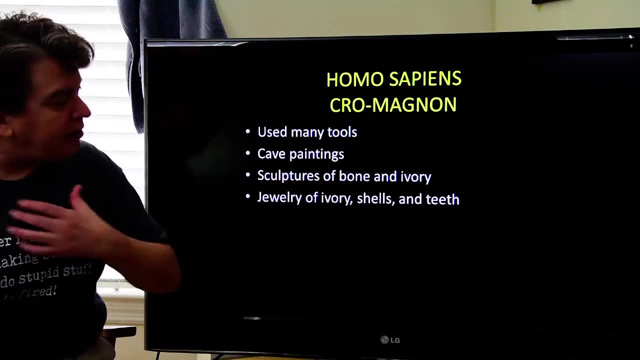 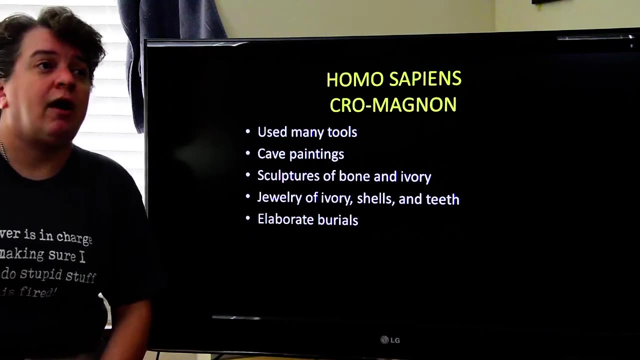 And they did have jewelry, And again the jewelry would involve, like ivory beads, that they would shape shells, teeth, and they would end up wearing these things, These things, as ornamentation, like necklaces. They did also have some sort of spirituality. 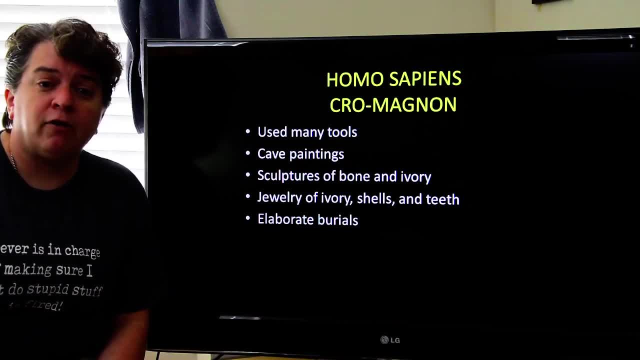 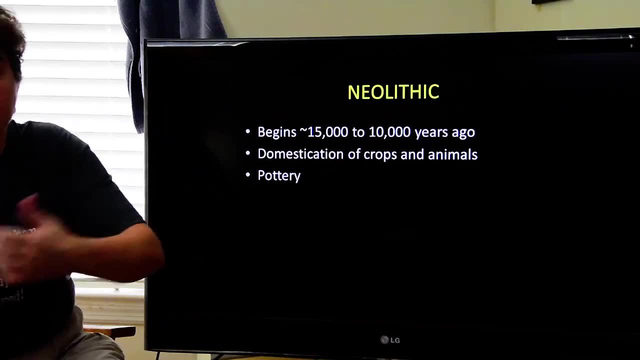 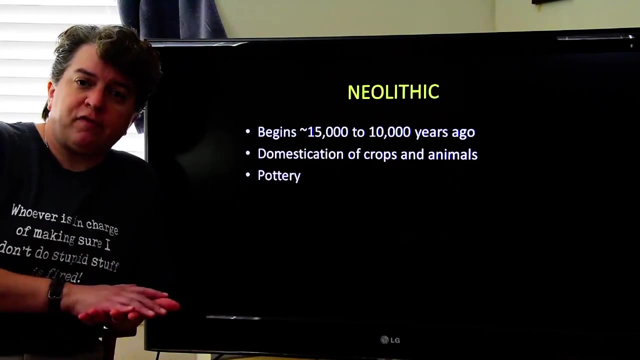 because they do have some fairly elaborate and complex burials. So when we are talking about early humans, when you study archaeology, you have these different time periods. You have the Stone Age, when tools were made of stone. You have the Copper Age, when people developed smelting. 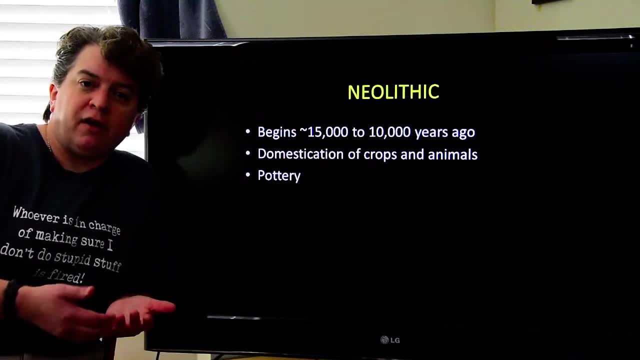 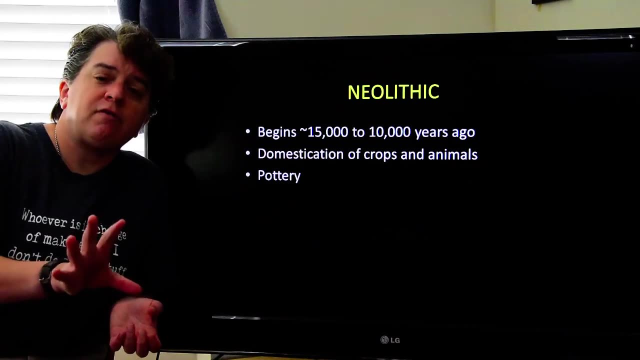 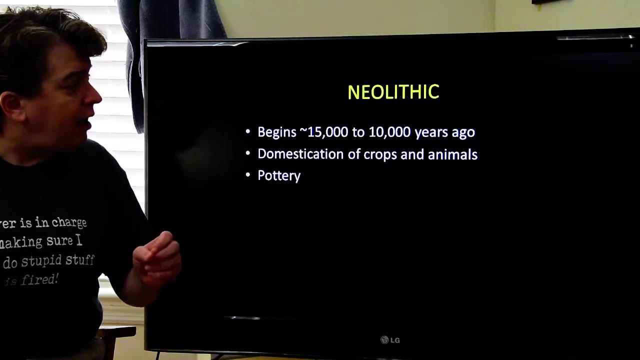 And started using metals, And you have the Bronze Age and the Iron Age, And so we are going to look at something very important that happened with humans all the way back in the Stone Age. The Stone Age is separated into three time periods, And that is the Paleolithic, Mesolithic and Neolithic. 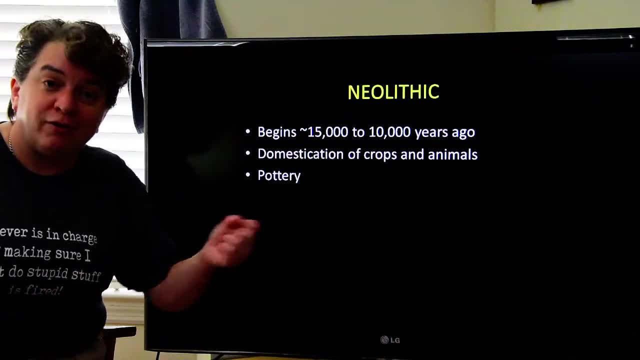 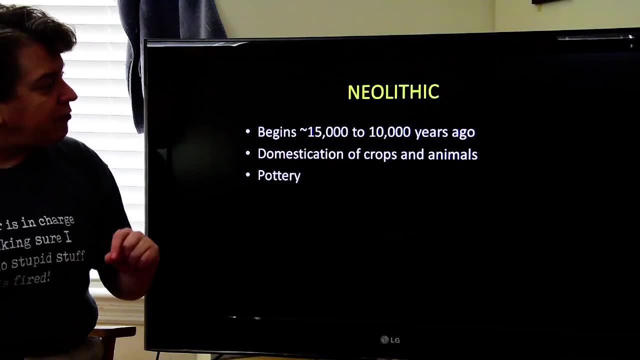 And so basically Old Stone Age, Middle Stone Age and New Stone Age, And we see some very important developments when we look at the Stone Age, When we get to the Neolithic. So the Neolithic begins about 15,000 to 10,000 years ago. 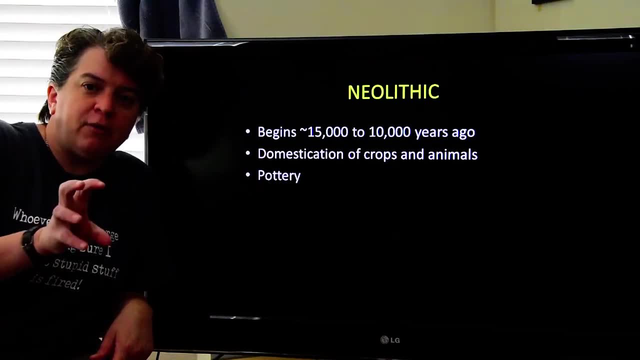 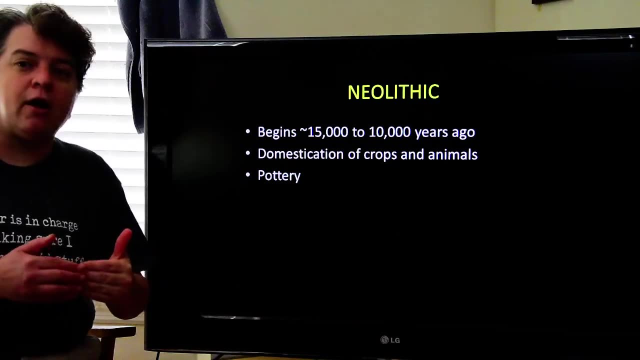 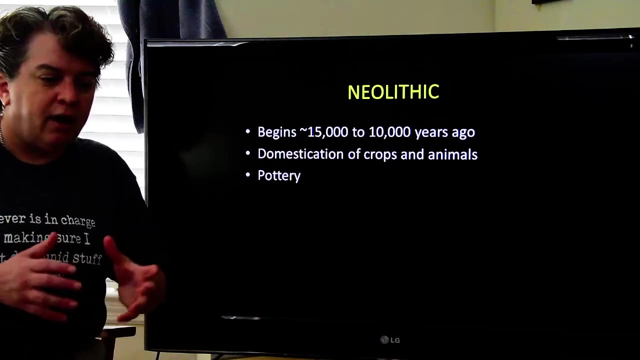 And the technological developments that mark this time is the domestication of crops and animals. So we are going away from just solely being these hunter-gatherer societies to actually growing crops instead of just wandering around looking for them, Just wandering around looking for edible things. 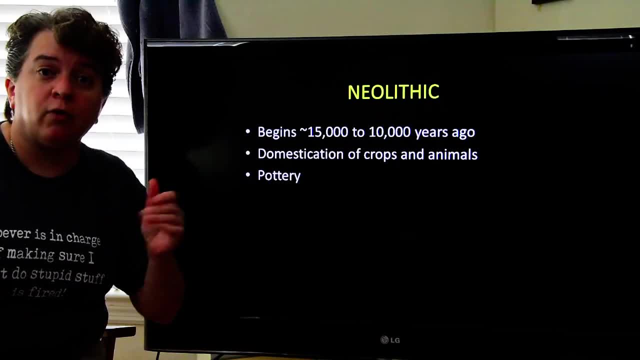 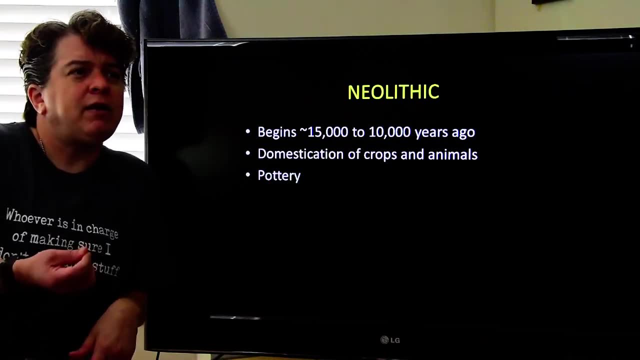 And also raising livestock instead of just wandering the woods trying to hunt for stuff. And so we have this domestication of crops and animals at this time. And so what they did? they would find things like. there is a grass called einkorn. 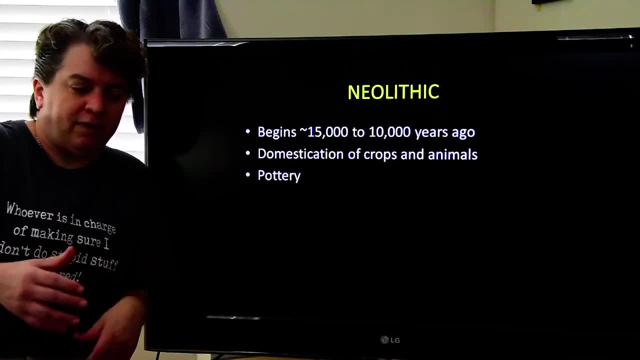 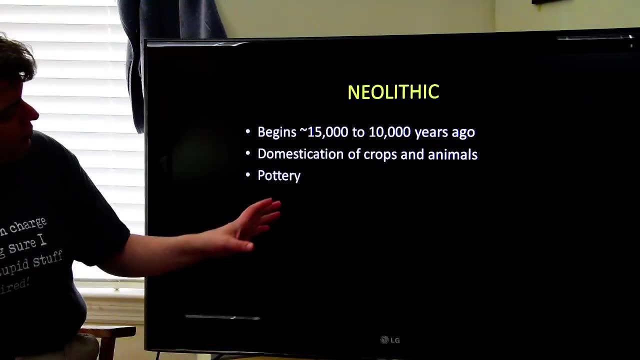 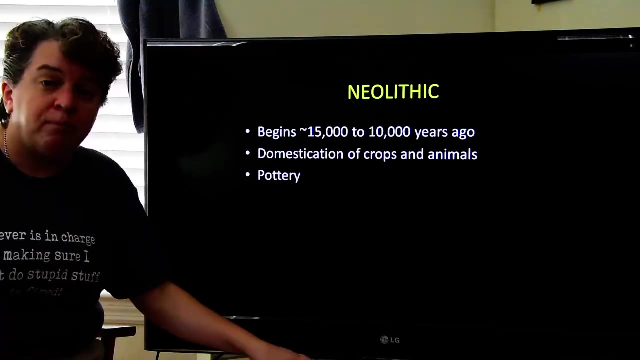 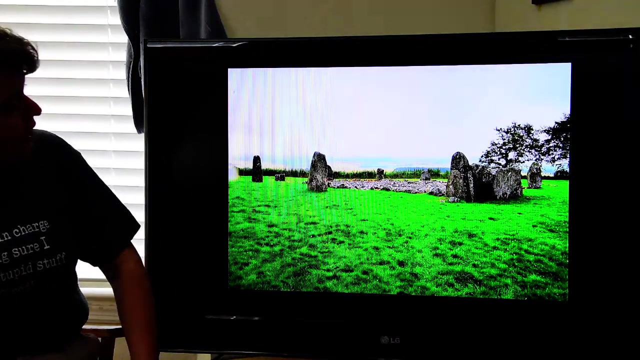 And instead of looking for that, they would start planting just entire fields of this einkorn And harvesting it and stuff like that, Now also in the Neolithic. another development we get is pottery. People start learning how to create pottery, And those are the technologies that define the New Stone Age. 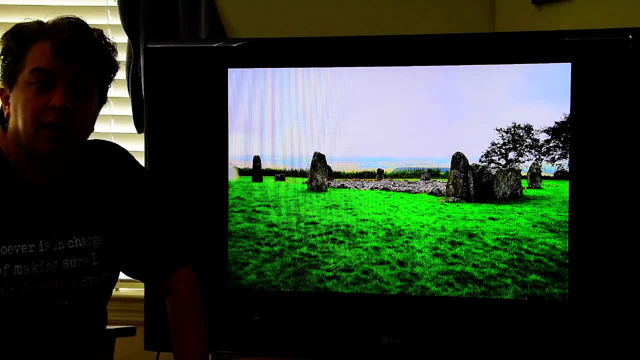 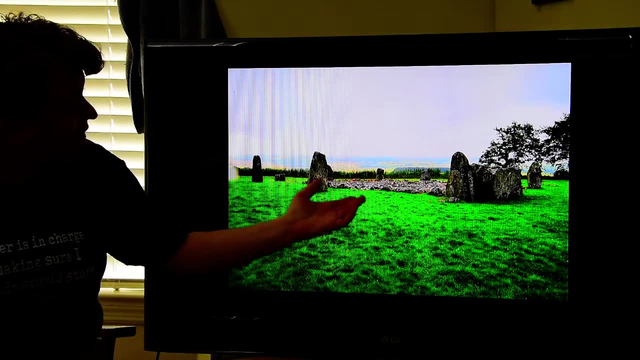 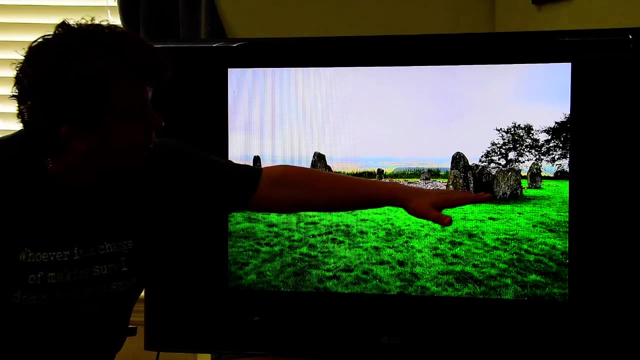 If you go to places, you might see some structures from the Stone Age, From the Neolithic Stonehenge or, in this case, this is another stone circle. up in Scotland This is called a recumbent stone circle- Recumbent because this stone happens to be lying on its side. 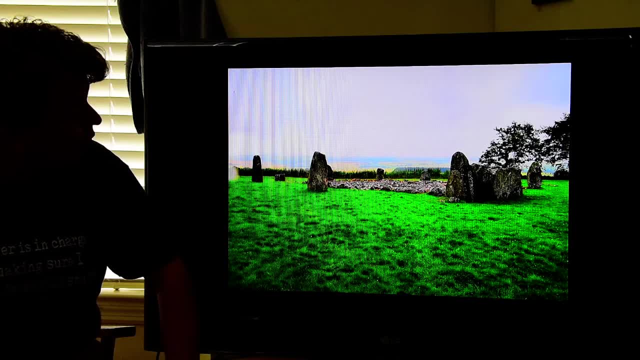 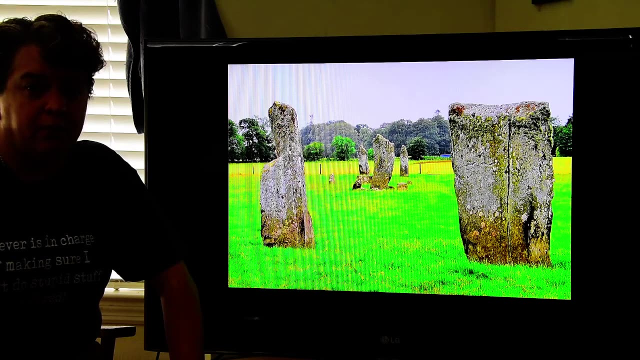 And it was purposely built that way. Recumbent stone circles were a ritual place where it seems like people did cremation burials, But you will see other standing stones in other places And we don't always know exactly what rituals were done with all of these. 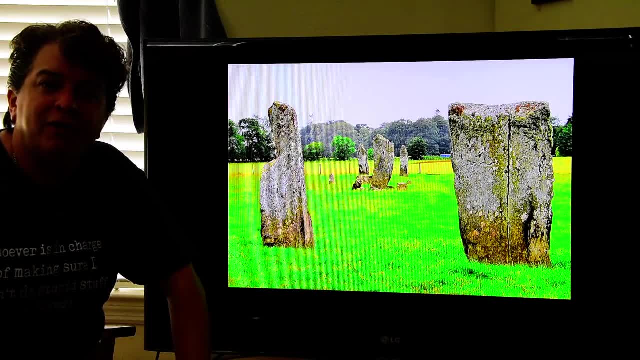 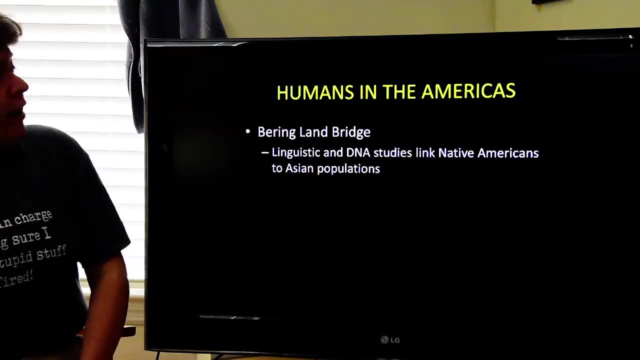 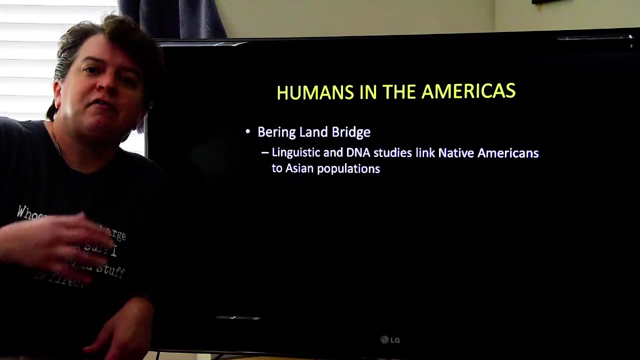 But anyway, these are some Neolithic monuments that have stood the test of time Because they are still there. Alright, but what about humans in the Americas? So far, everything I have been talking about, we have been looking at like East Africa or Eurasia. 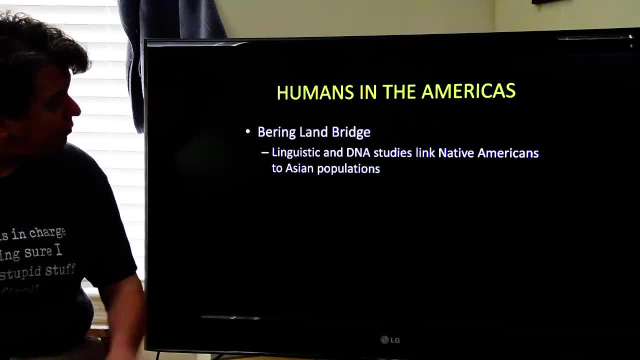 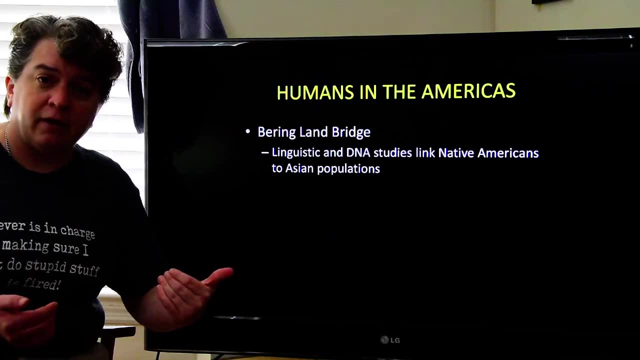 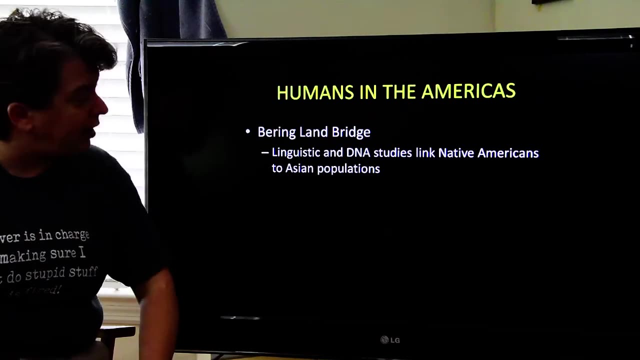 Well, we do get humans in the Americas, And they came here across the Bering land bridge. So during the Ice Age, sea levels were significantly lower And so up in Alaska. basically, Alaska and Northern Russia were connected by this Bering land bridge. 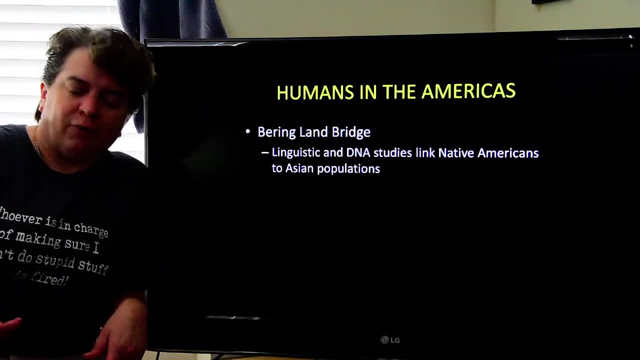 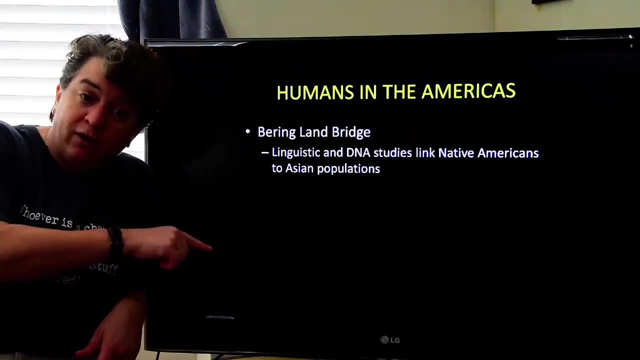 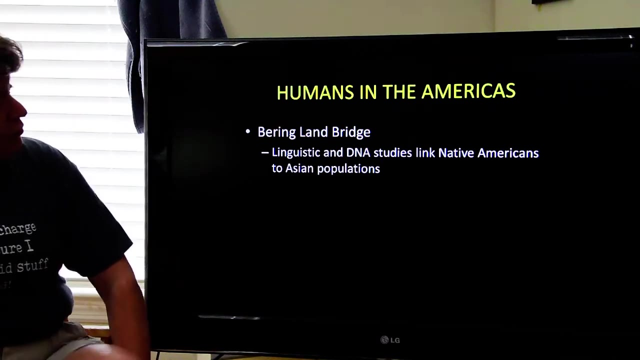 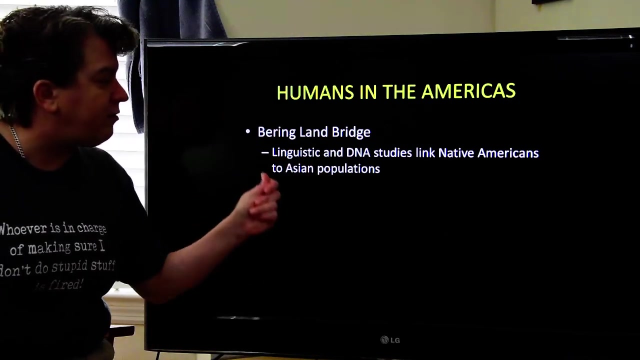 And animals migrated across that. We had things like camels headed into Asia, Camels and horses and stuff. But we also had humans coming from Asia into the Americas And when we do studies of this, linguistic studies and DNA studies link Native Americans to Asian populations. 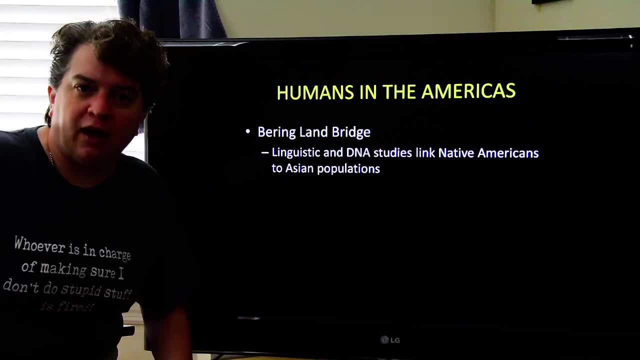 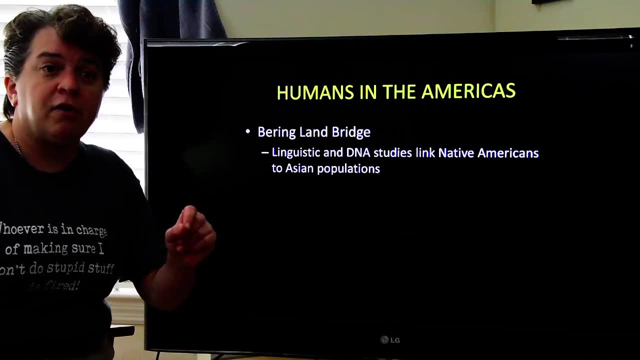 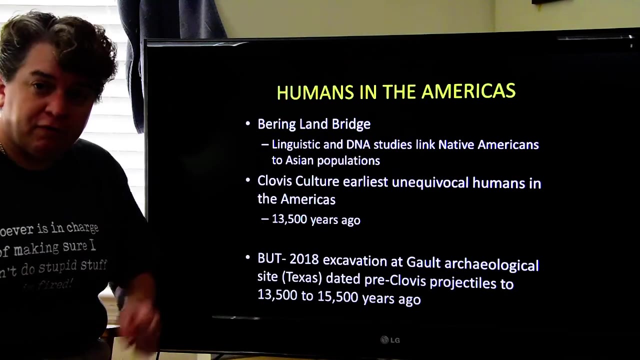 So it's not just that it seems like that's how it happened. There are real hard evidence that, yes, the Native Americans ended up coming across that land bridge from Asia. Now, the Clovis culture is an important culture to remember when we are looking at. 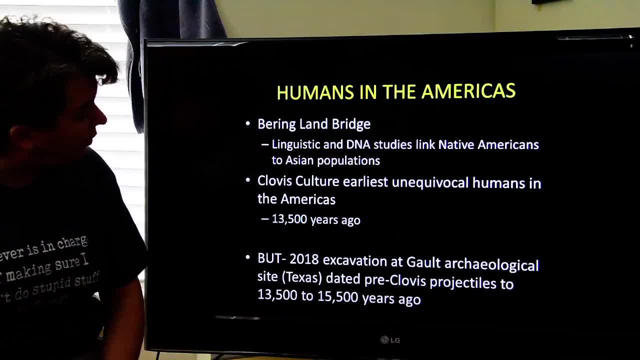 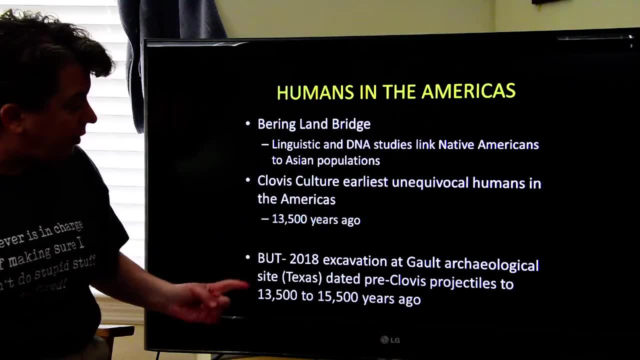 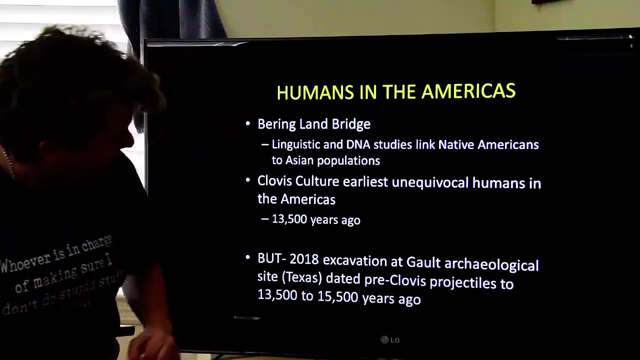 the settlement or population of humans in the Americas. This is the earliest unequivocal, meaning no arguments about it, of humans in the Americas at 13,500 years ago. But but wait, there's more. In 2018, there is an excavation right here in Texas. 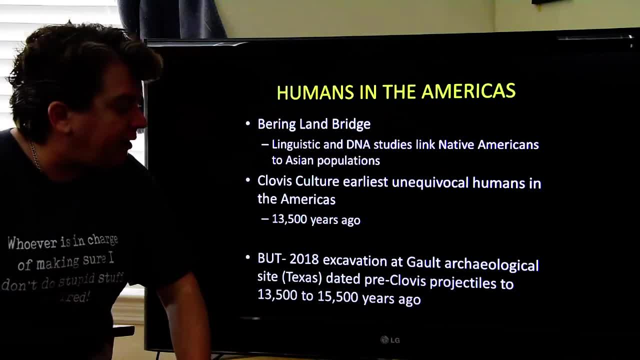 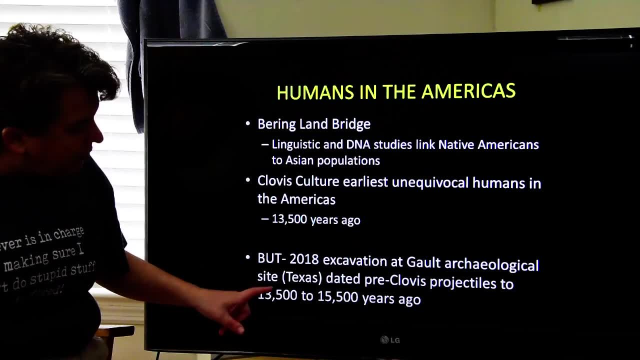 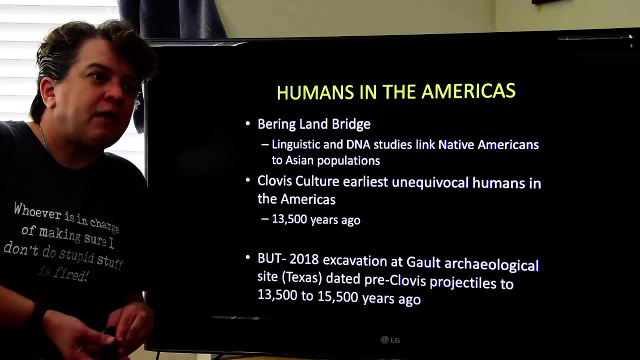 at a place called the Galt Site And this dated some pre-Clovis projectiles projectile basically spear points to 13,500 to 15,500 years ago. So what that's telling us is that people might have been living in the Americas longer. 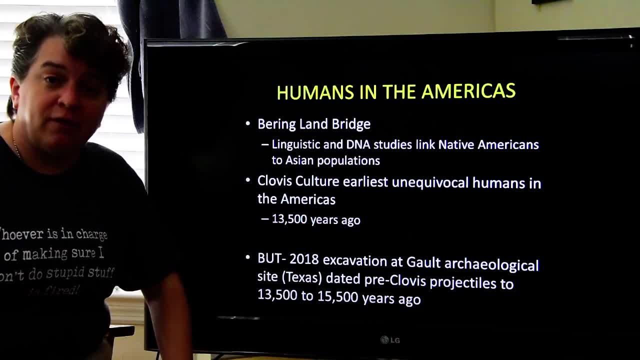 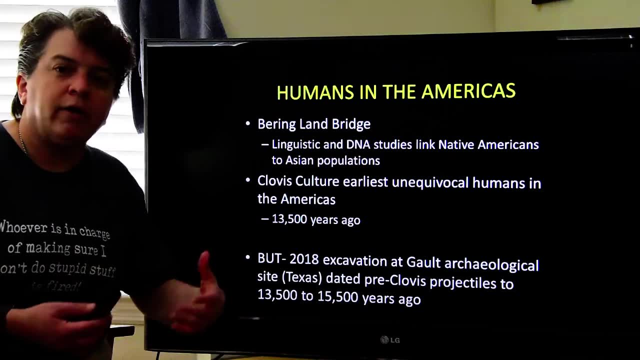 at least a little bit longer than we've previously thought, And I always try to give you guys, when there's new research or ongoing research, I always try to make sure to include that, And so this is kind of one of these very interesting things. 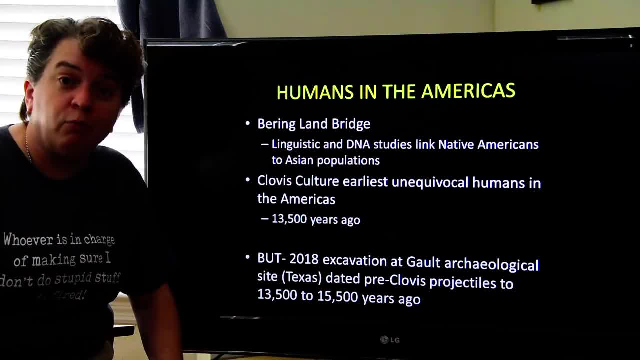 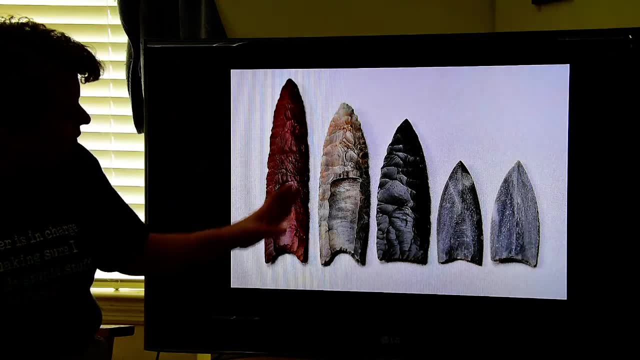 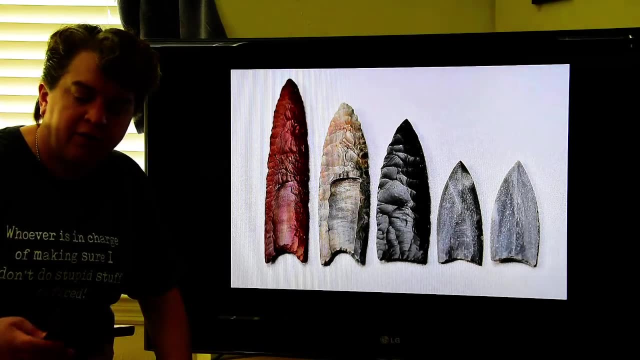 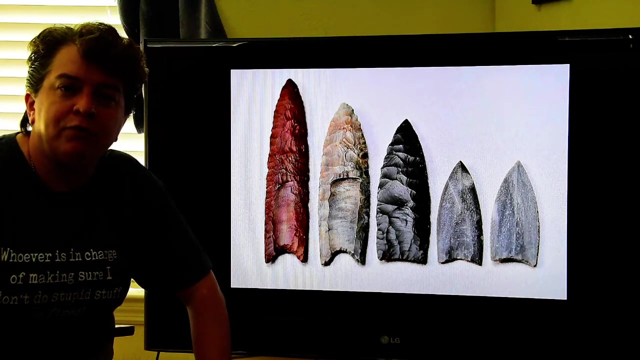 that warrants more study. Now these are Clovis projectile points. They're very nicely designed. You would attach it to a spear or here and use that for hunting some of the woolly mammoths and mastodons and bison and stuff that occupied North America. 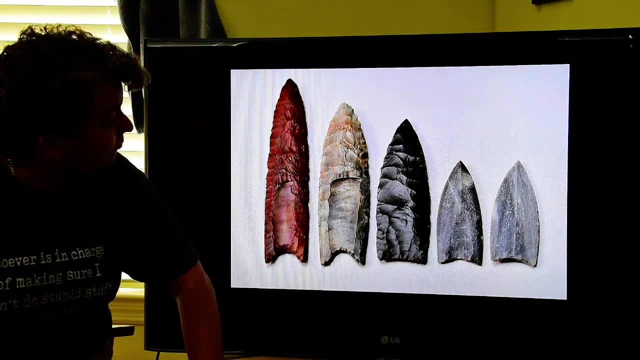 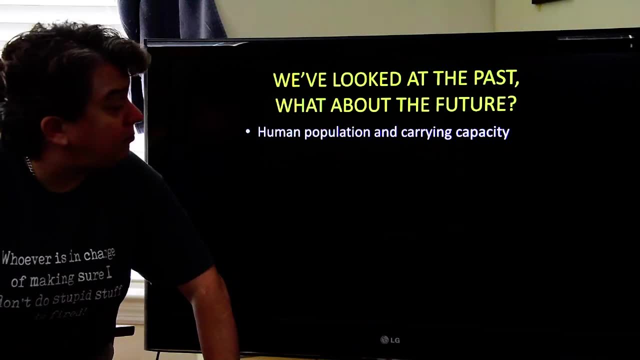 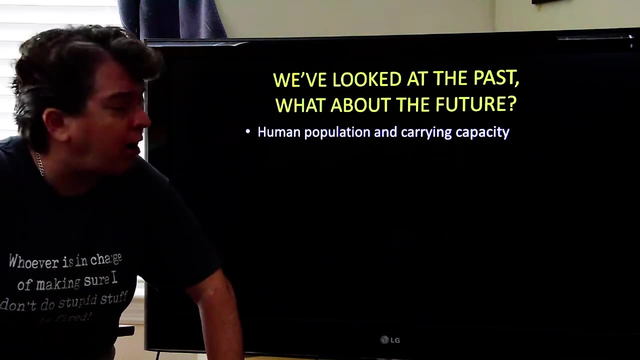 when these hunters, when these hunters, traveled here. So we have spent, then, this past semester looking at the past, right, Looking at how Earth formed and how it has changed over time. But what about the future? right, We've got to think about the future. 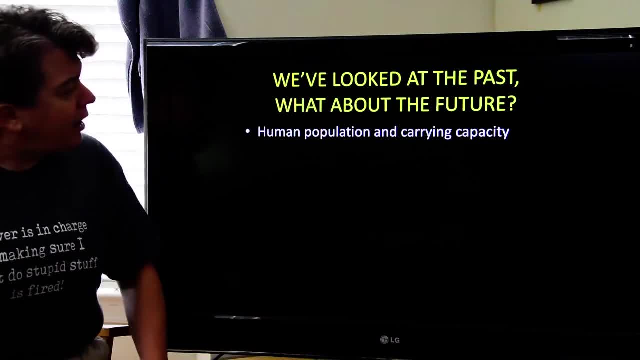 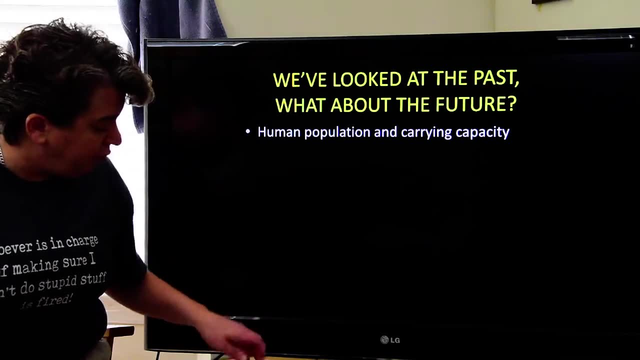 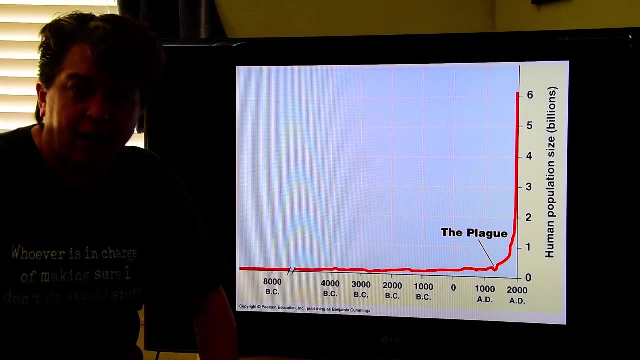 and where Earth is heading from here, And one of the things that's important to consider is the carrying capacity of our planet and the human population. Now, I don't want to sound like Thanos here or anything, but all planets have a carrying capacity. 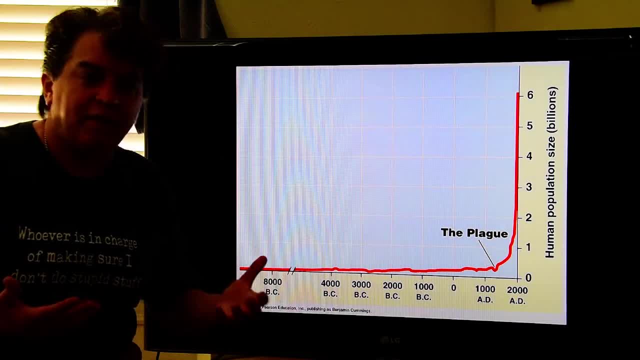 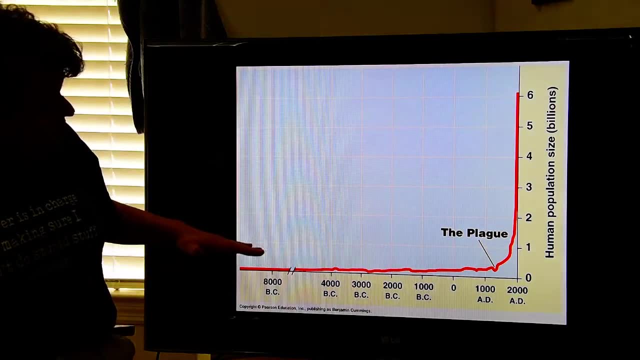 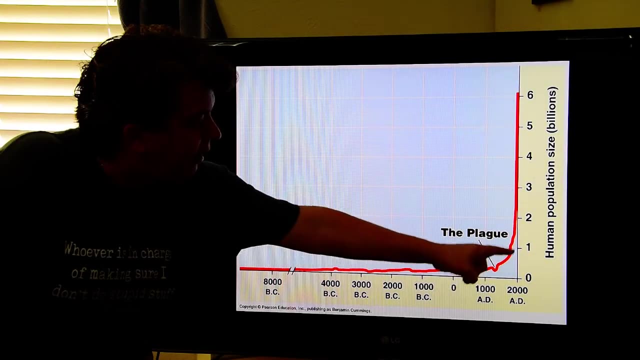 a certain amount of population that they can support, And what we're looking at here is from 8000 BC to 2000 AD. the population of people on the planet- And you can see that it has there's Black Death- it has skyrocketed. 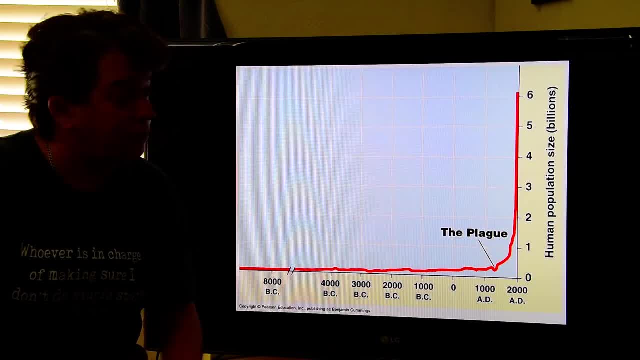 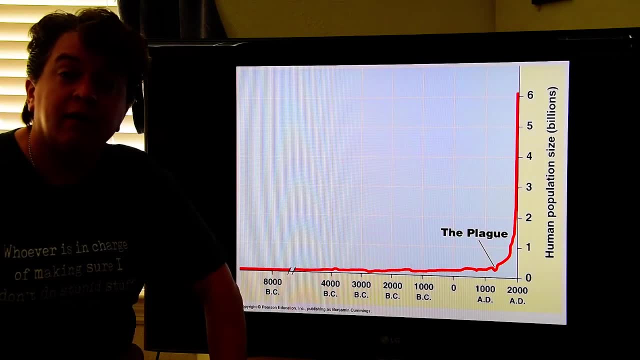 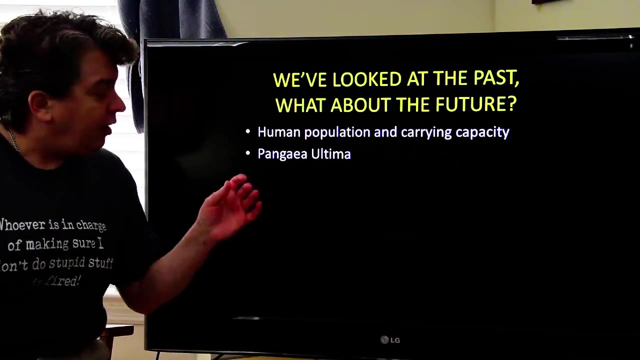 And the question is: how long can this planet's resources sustain this many billions of people on the planet? And that is something that should be considered when we look at the future. Now, what about plate tectonics in the future? Well, the plates are going to continue moving. 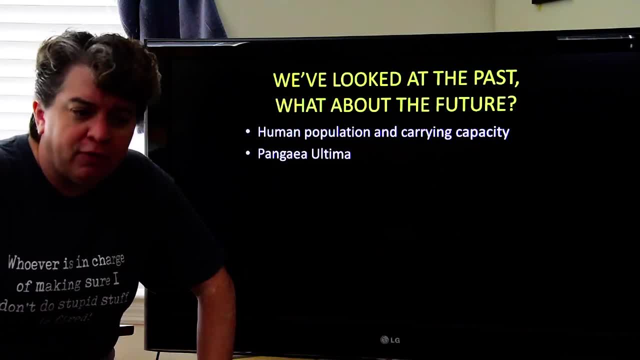 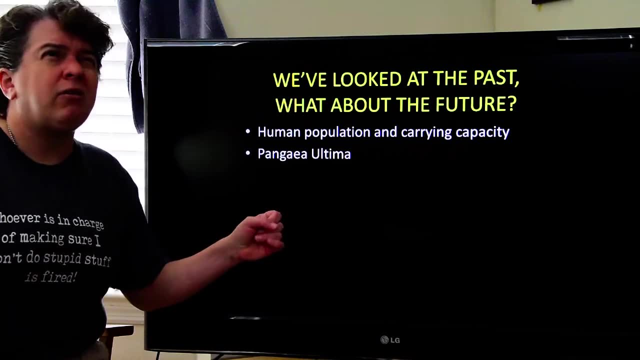 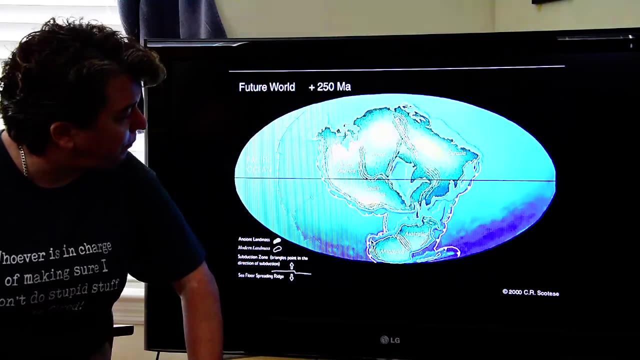 and if they continue moving the way they are now- and we can kind of estimate what will happen In about something like 250 million years, we're going to get Pangea Ultima, our next supercontinent, And that's what it's going to look like. 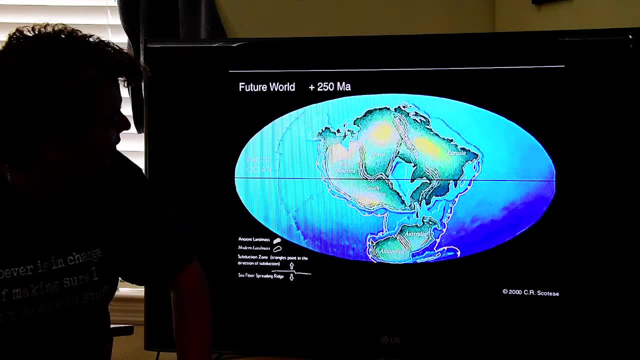 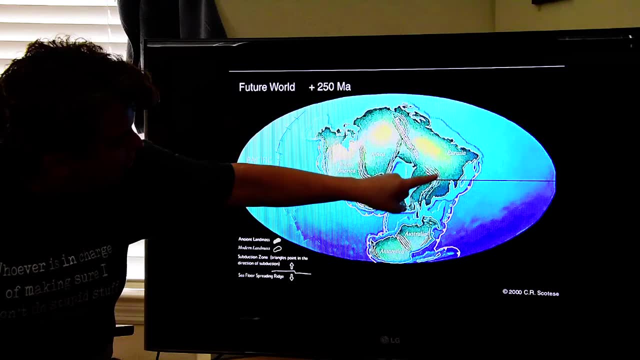 At least that's what we're hypothesizing. our next supercontinent's going to look like. We've got North America, South America, Africa. This is like Europe and Asia and Antarctica And Australia. If you want to see this, go into YouTube. 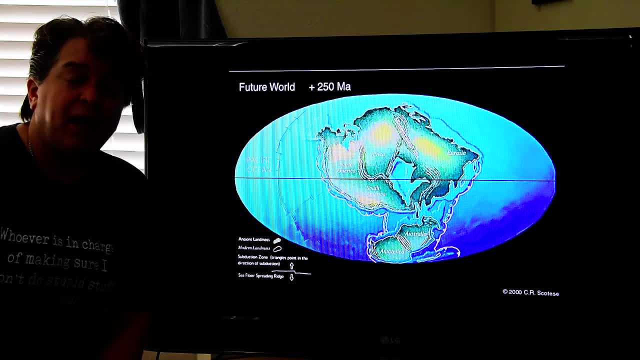 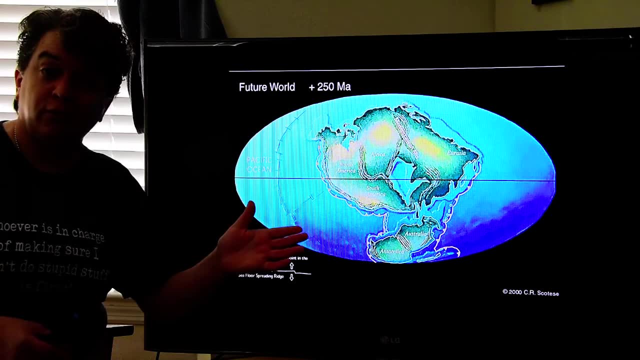 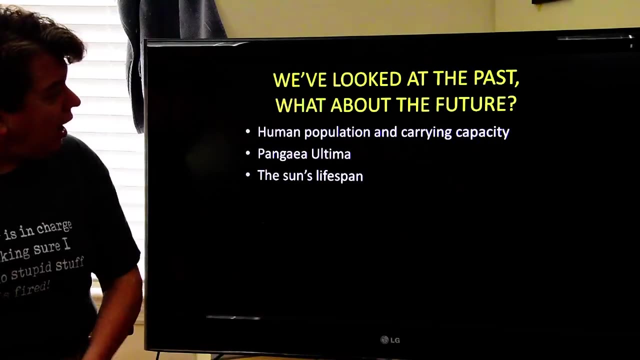 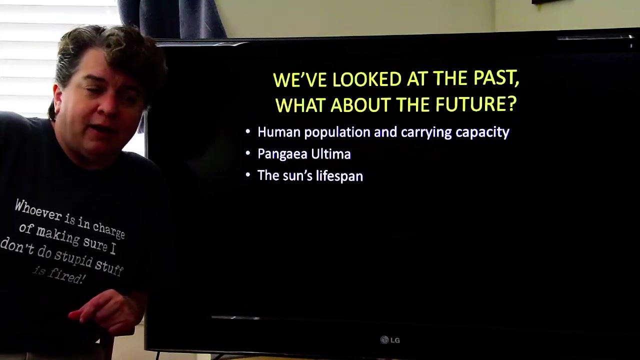 and basically, in the search bar, simply type in Pangea Ultima and you will get a YouTube video that's going to show you how the plates are going to move over the next 250 million years. Now, the other thing about the future is the sun's lifespan. 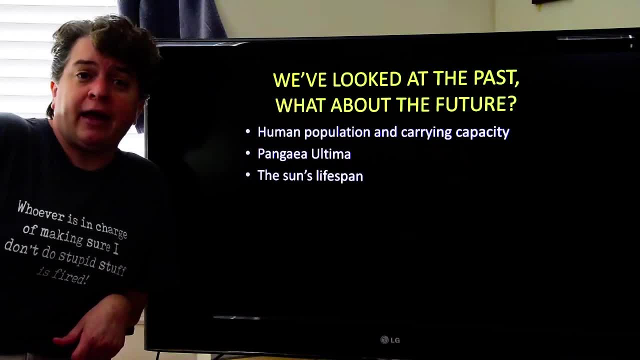 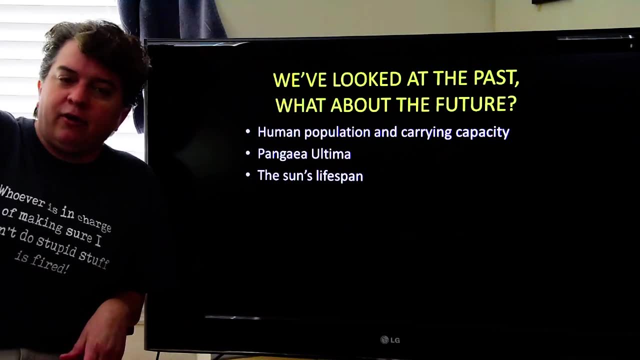 Stars don't last forever and our star is middle-aged- It's kind of at the prime of its life, shall we say- And it's been happily doing fusion and giving off energy for the past 4.5 billion years and it will probably last another 4.5 billion years. But then it is going to transform into a different type of star, and when that happens, either Earth is going to be consumed by the new star that the sun will become, or Earth might be kicked off into the depths of space. We're not sure, but either way. 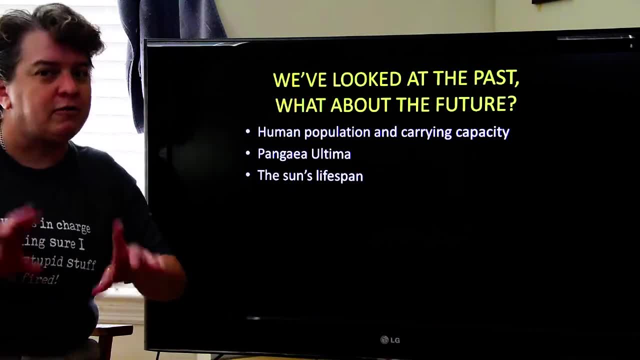 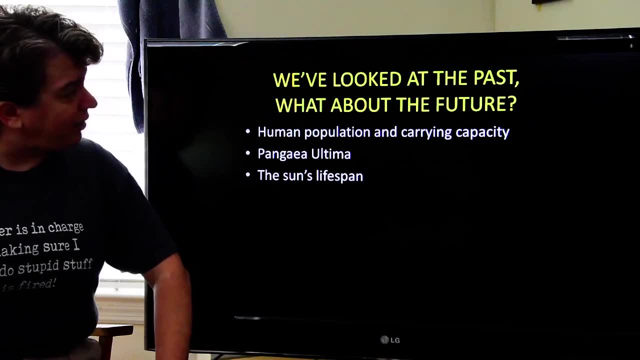 it's really not going to be good for our planet, But you don't have to worry, because that is 4.5 billion years from now. So this is some of the future to look at And the random picture of the day, since this is the last lecture. 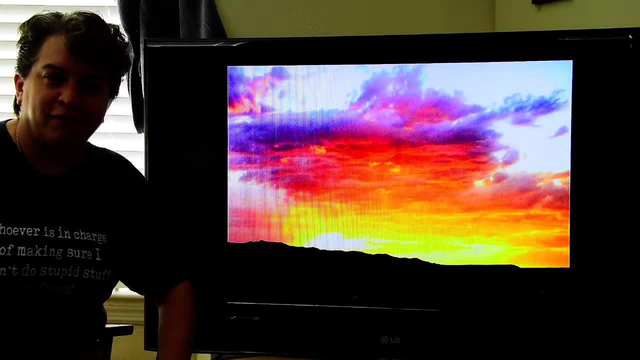 is a sunset, We shall ride off into the sunset together.